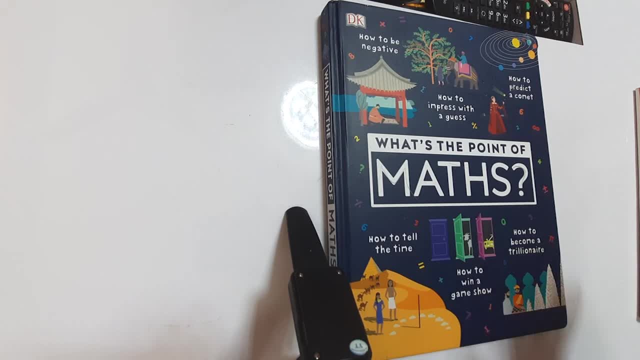 If you all think that maths is difficult, let me tell you, if you go through this book, then you will find maths to be super easy. So in between, when I'm telling you stories every now and then I will also be teaching you about these kind of quiz and puzzles and all. 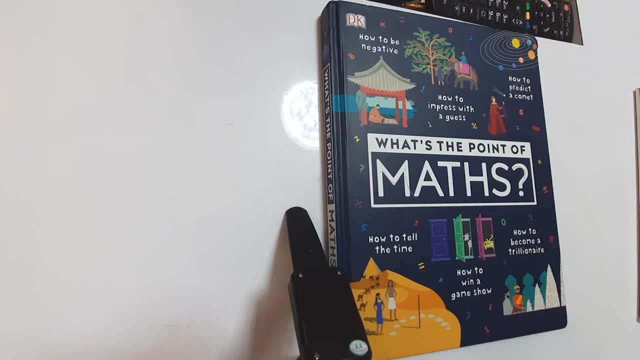 related to maths And it's going to be so much of fun that you're going to fall in love with maths. Yes, of course, And that was Tushar. Okay, Now, the name of the book is: What's the Point? 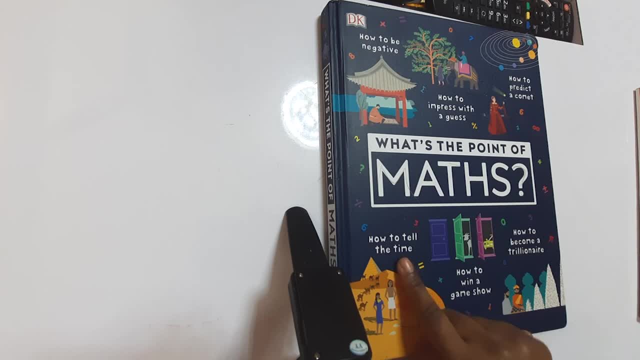 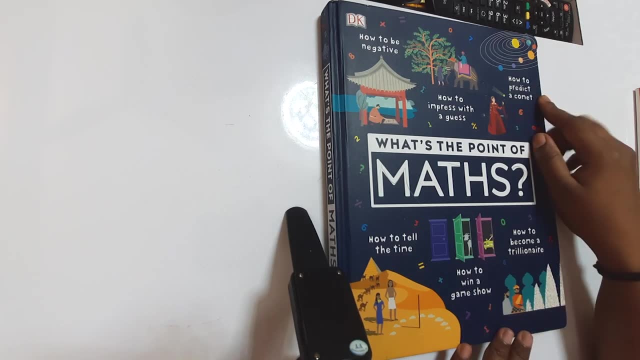 of Maths. So this book is going to teach you on how to tell the time, how to win a game show, how to become a trillionaire, how to predict a comet, how to impress with a guess and so many things. Okay In case, if you're ages six years or more, then you should definitely buy this book. 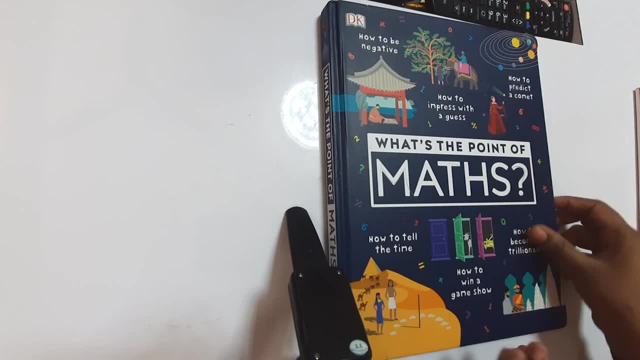 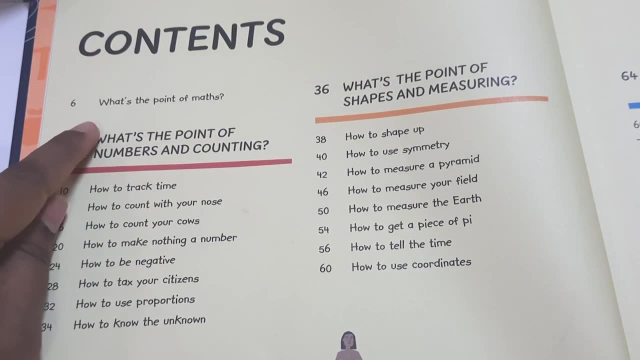 And you should try the things which are given in this book. Okay, So in the contents, let me just show you what all this book has. So this book has got. what is the point of maths? Why is that we need to learn maths And why do we? 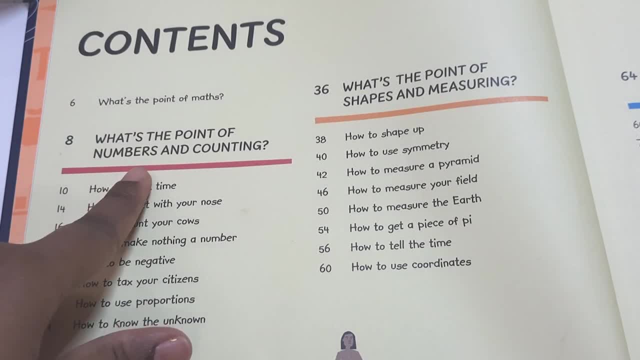 need maths in our life And it is also going to tell us what is the point of numbers and counting. You know, as soon as you started joining the school and all the very first thing, the teachers thought you were counting numbers from 1 to 10, correct, And you were learning 1,, 2,, 3,, 4, like. 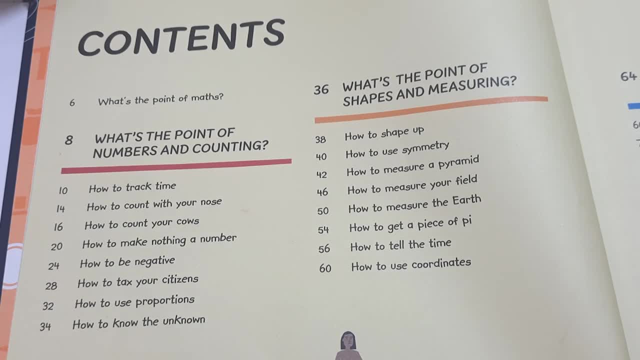 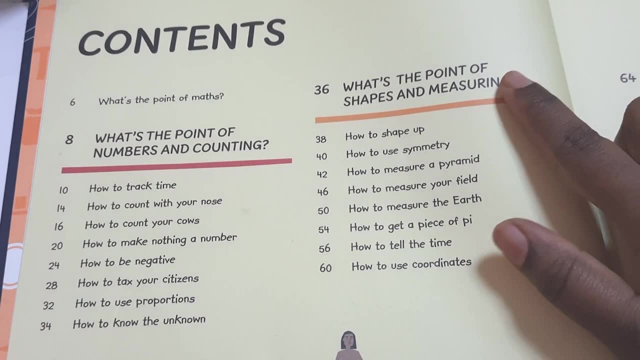 that you were learning until 10.. But what is the point of numbers and counting? Why should you know all these things? So this book is going to teach you that, And this book is also going to teach you what is the point of shapes and measuring. Why do you need to learn the shapes and how to measure the shapes? Why do 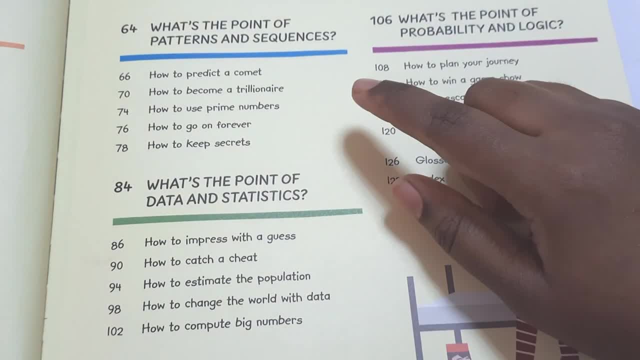 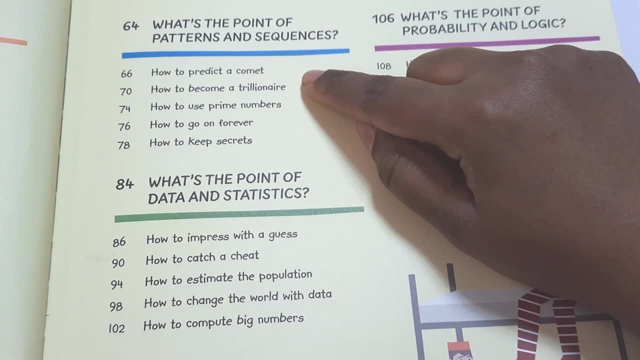 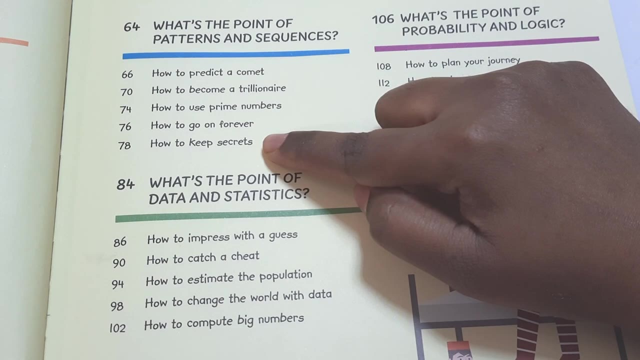 we need shapes. Okay, And not just that. this book is going to teach you the point of patterns and sequences, Like: how do you predict a comet, Why do you need prime numbers, How do you go on forever And how do you keep secrets? Oh my god. 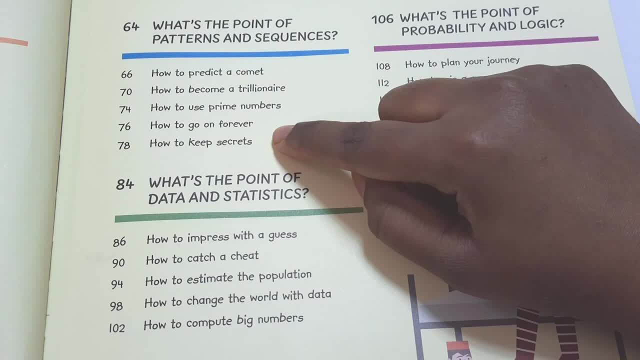 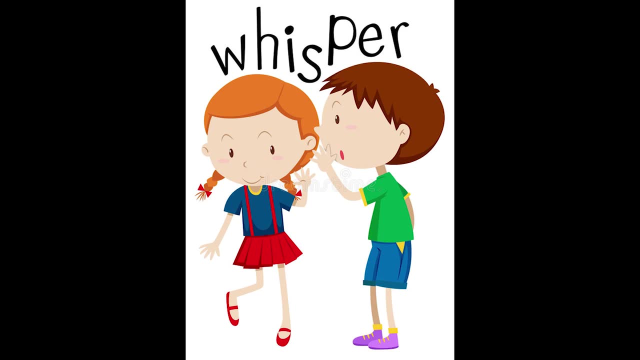 This book is going to teach you how to keep secrets and how to talk to people in a secret language. Isn't it exciting- And this is what I will be teaching you today- And it's going to be so fun that you can talk to anybody you want in a secret language and nobody will know what you're. 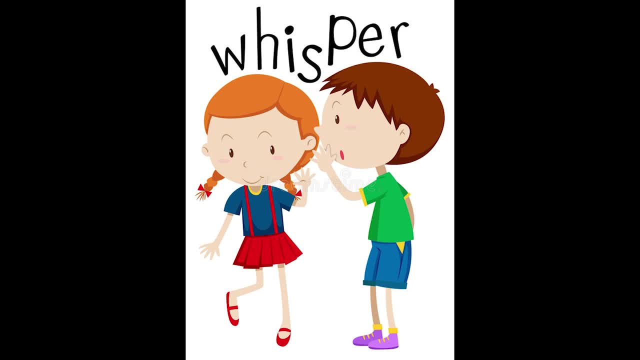 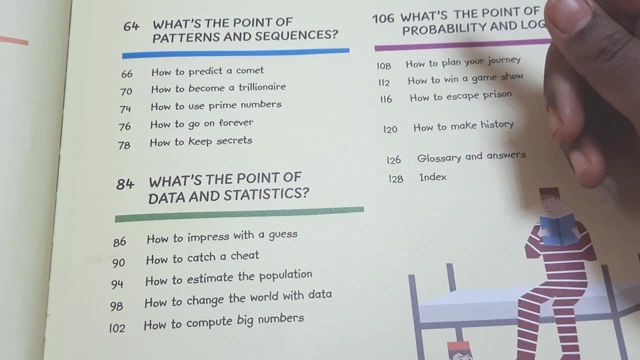 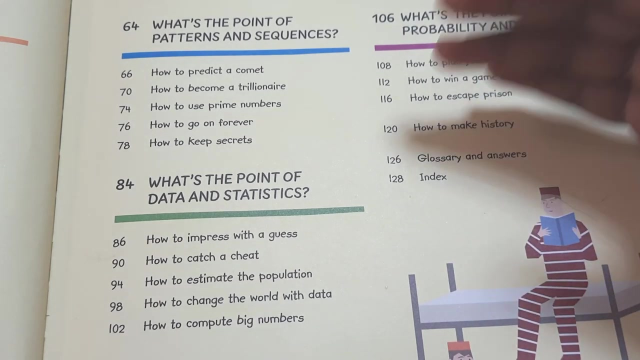 talking about. Imagine that you can send any message you want in WhatsApp And even if your parents happen to see that message, they will not understand what message is it what you're sending? and all So exciting, right. And this book also teaches what is the point of statistics, like how to impress with a guess. If you want to impress somebody and you know there is a very big puzzle which is being given to you, or a big choice that is given to you- Like, for example, there will be three doors and you are asked to choose one of the three doors, Okay, And you want to guess in which door will there be a thing which is most interesting to you or something that you love? So how will you guess which door it is that you need to choose? 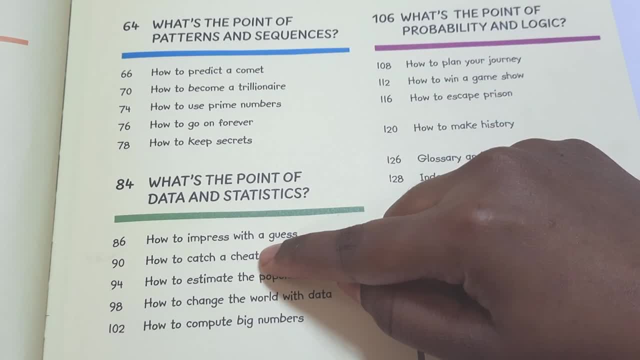 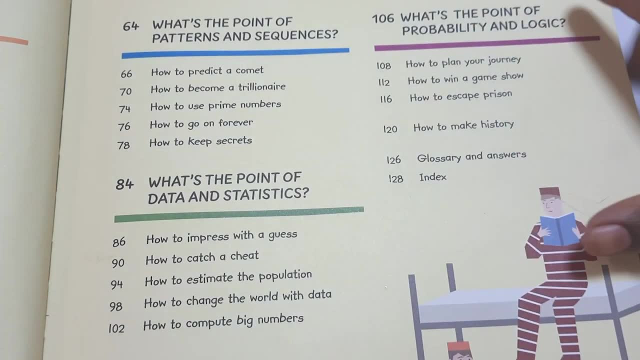 So this book is going to help you with all that, And this book will also help you catch a cheat, in case, if you're playing a game, then how will you catch a cheat? So, like that, there are many more things that you can learn with this book, And it is super simple. Any child can understand how to read and you know how to understand all these concepts, Okay. So, in case, if you don't have this book, tell your parents to get you this book. This book is available on Amazon. Okay. 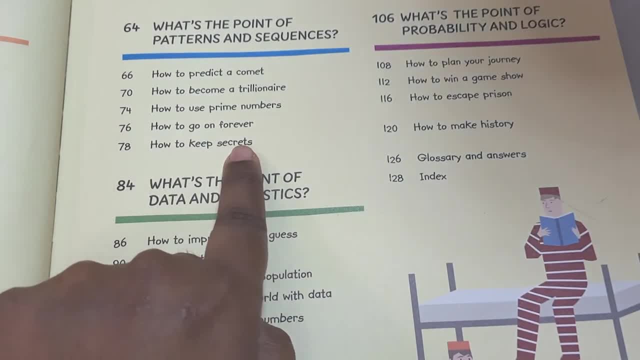 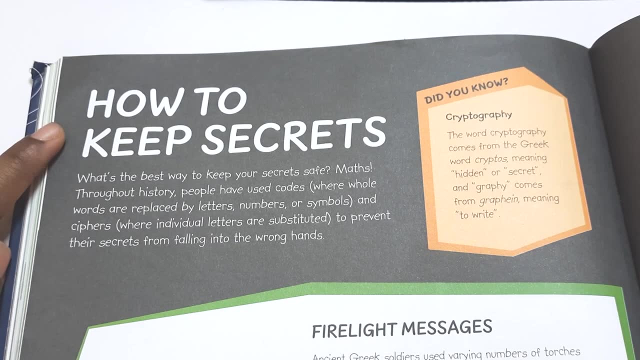 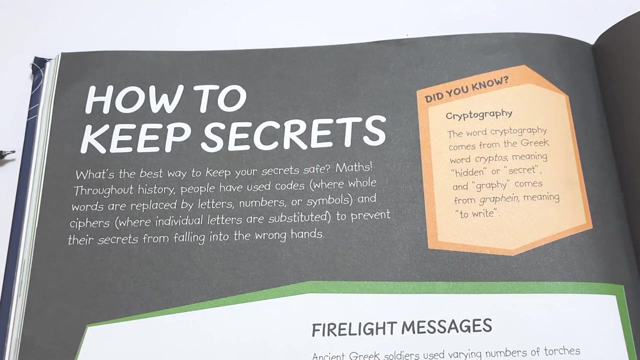 Now let me just go straight away to this place where it says how to keep secrets. Okay, so here it is, how to keep secrets. Let me just read what is written over here. So, my dear children, how do we keep secrets? What can help us in keeping secrets? 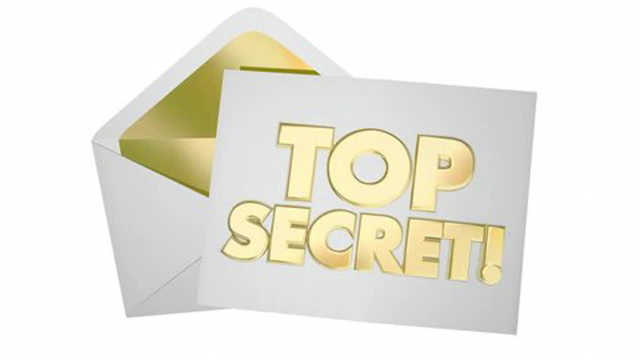 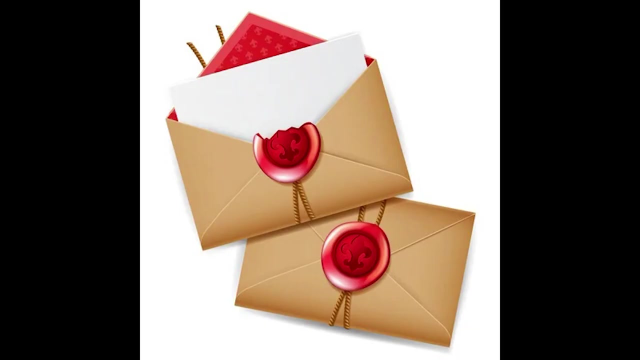 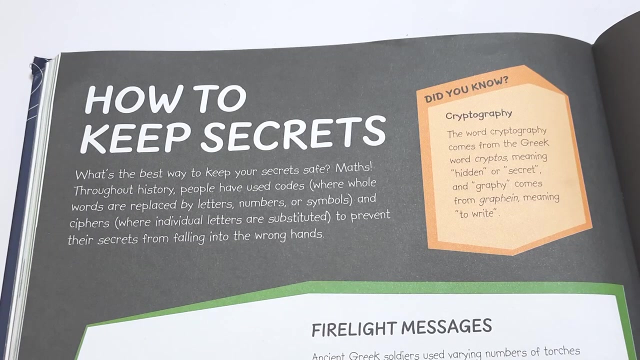 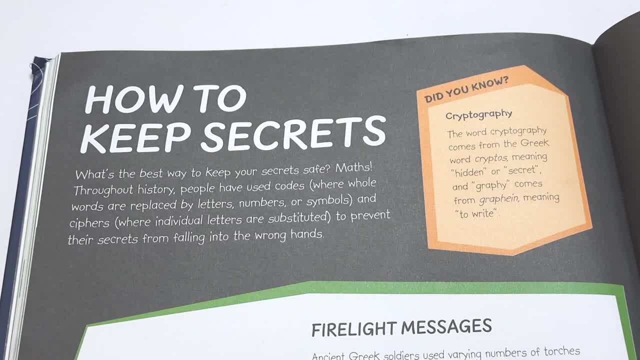 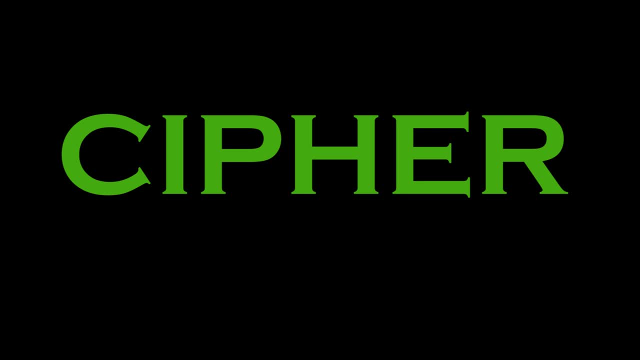 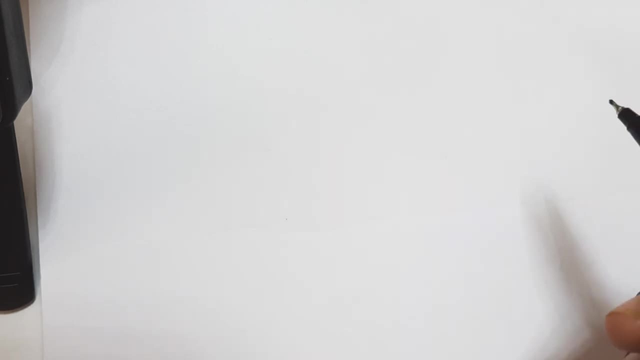 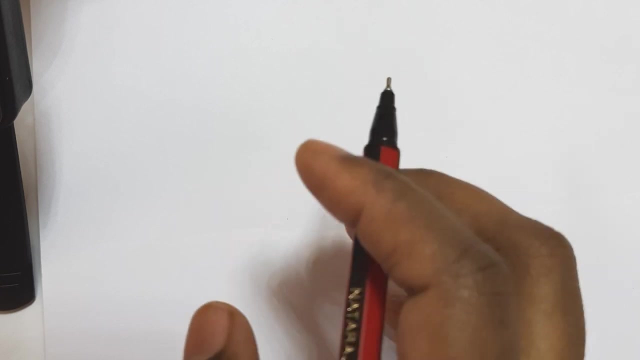 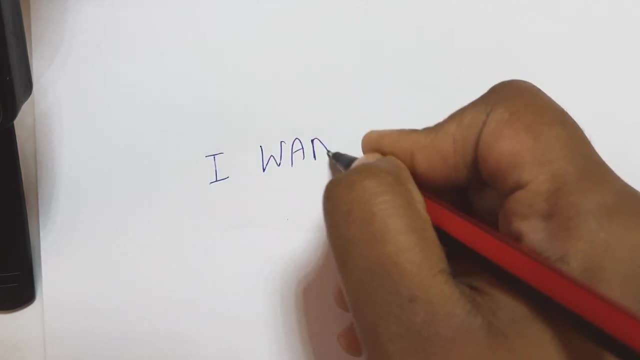 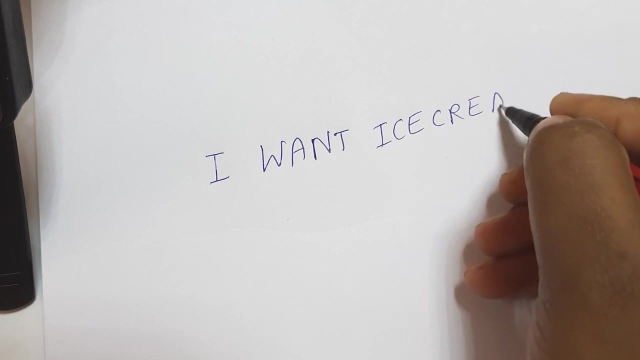 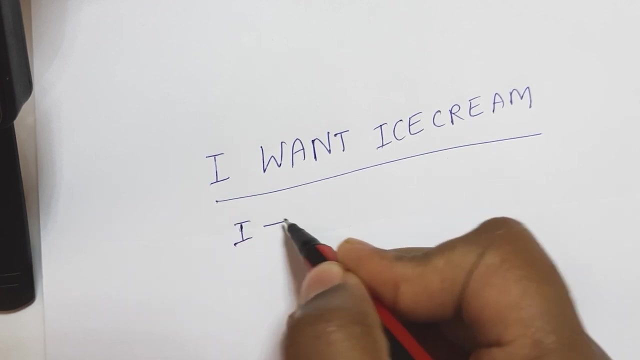 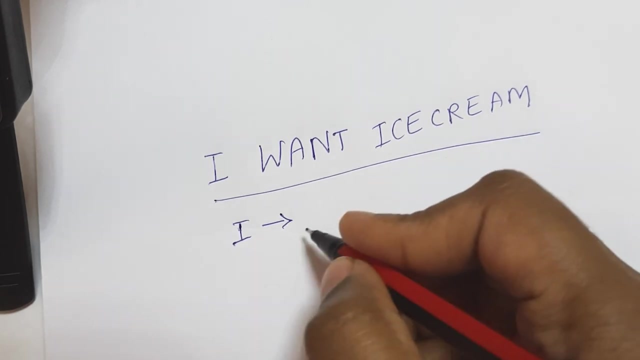 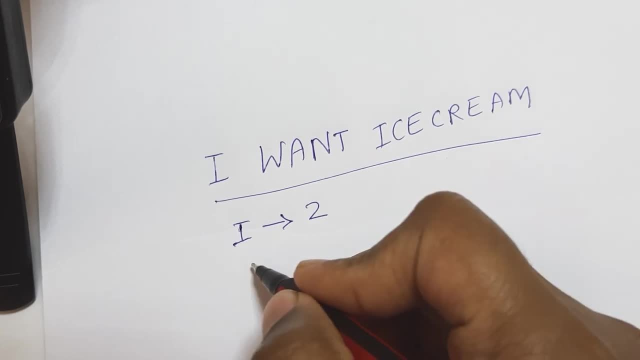 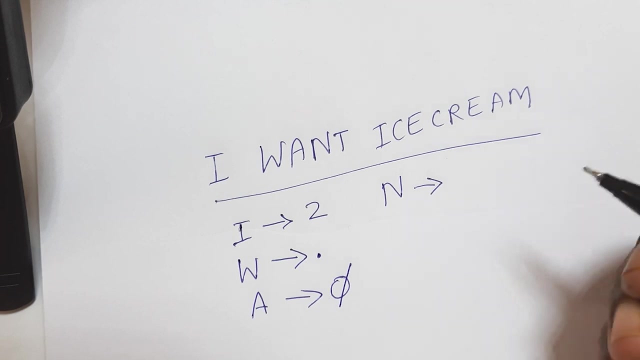 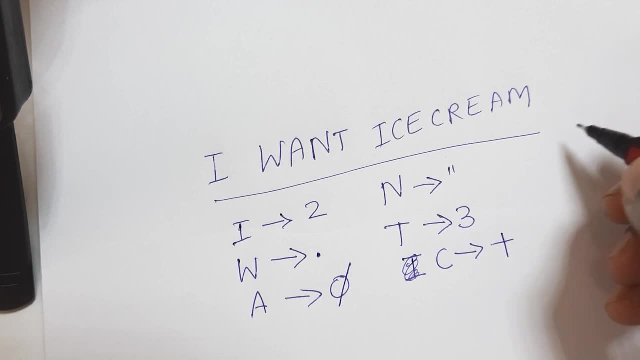 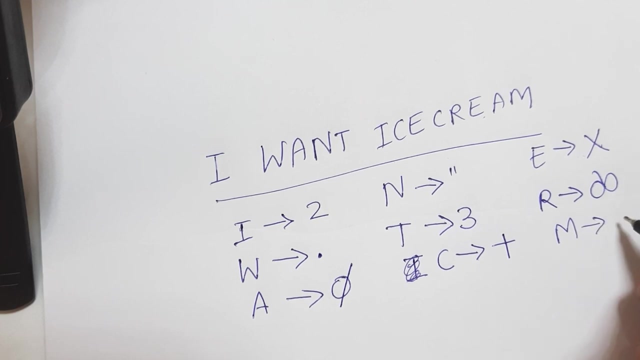 the symbol plus. okay, E I will be replacing with X. okay, X as in into mark, which is there for multiplication. okay, then R I will be replacing with, let us say, infinity. okay, and then we already have something for E. we have covered A and M, so for M, I am going to give number 9, okay, so now? 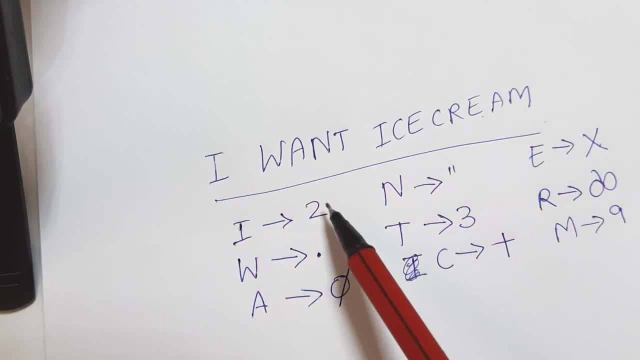 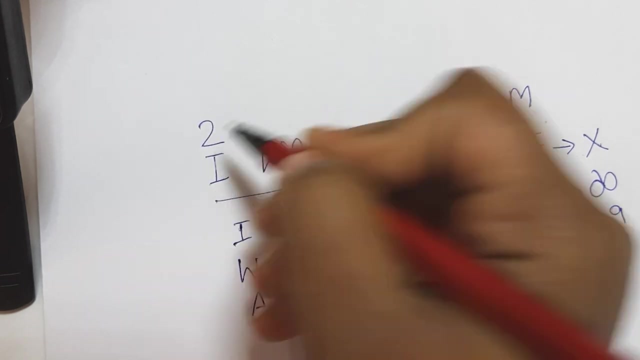 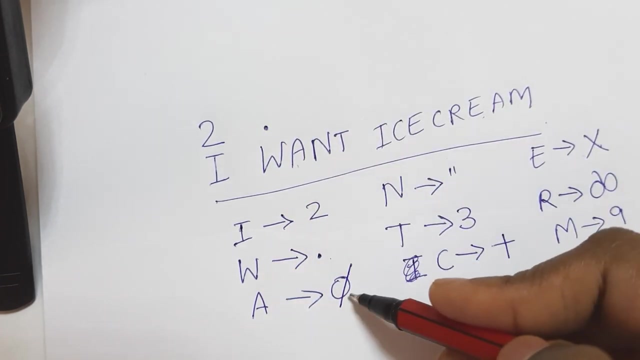 let me just write the same sentence using by replacing these alphabets with the corresponding numbers of the symbol. now, instead of writing I, what do I need to write? I need to write 2 right now. instead of W, I, I need to put a dot and instead of a, I need to write this symbol. instead of n, I need. 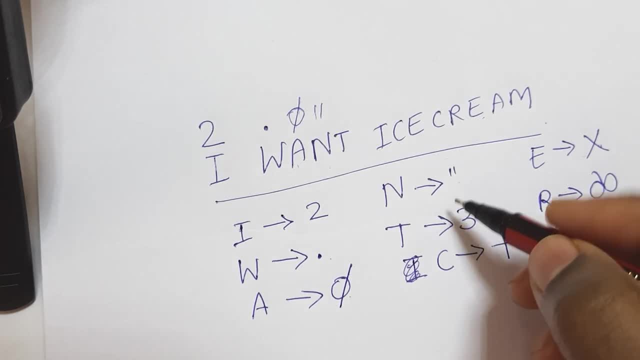 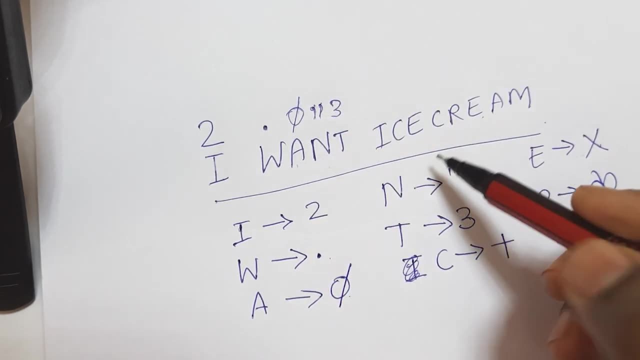 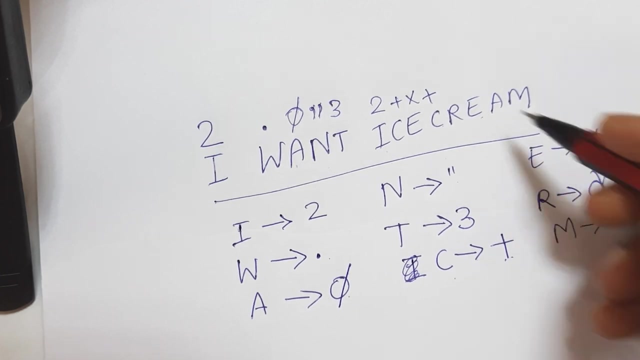 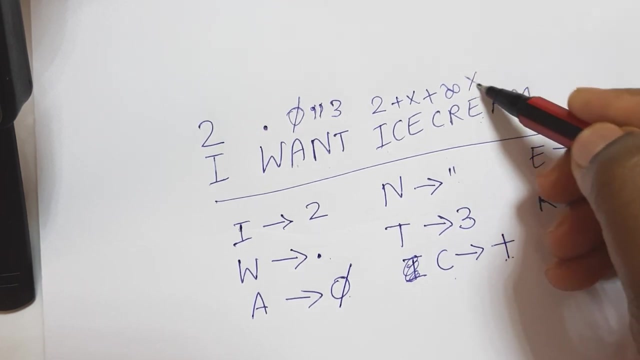 to write double quotes, and instead of t I need to write 3, and instead of i I need to write 2 again. instead of c, it is plus. instead of e, it is x, then again c, it is plus. then we have r, which is infinity, then we have e, which is x again, and then we have a, where 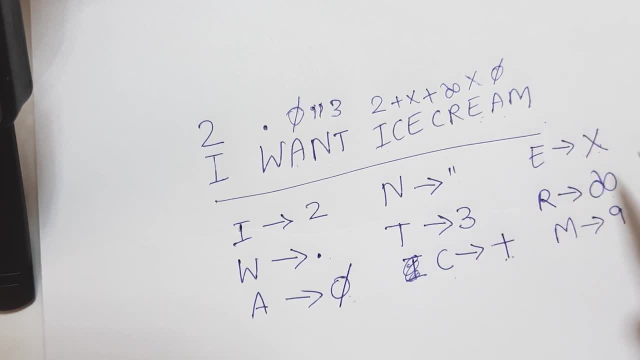 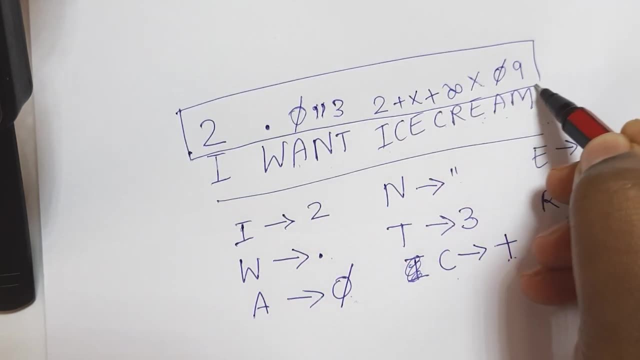 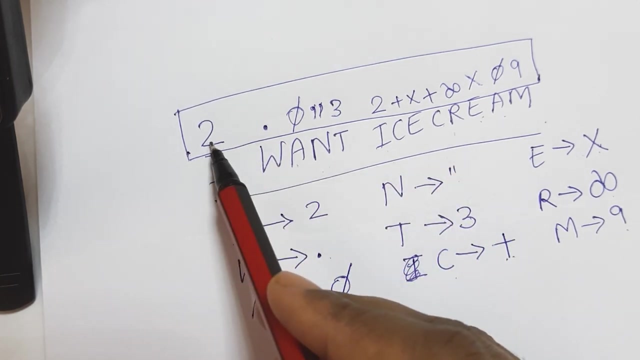 we have to write this symbol, And then we have m, where I need to write 9, so I will be sending this message to my friend instead of sending I want ice cream. Now tell me who can understand, looking at this, that I am sending a message asking for. 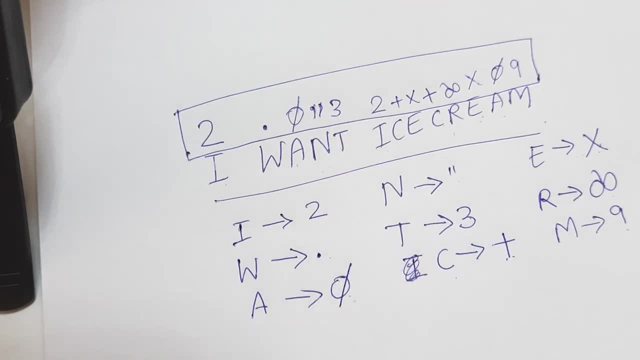 an ice cream. nobody can find that out right. but do you know, children? how can anybody read this? How can your friend read this and understand what you want? He can only read it if he knows what is the replacement for each and every letter like. 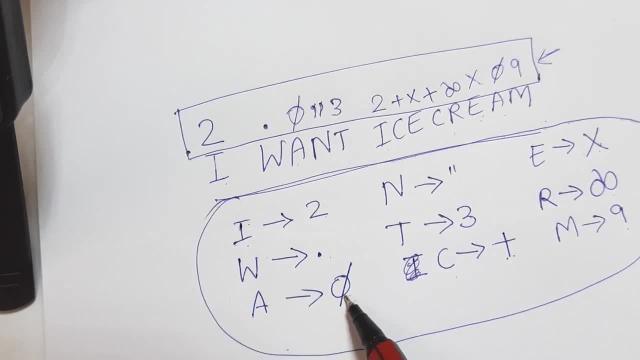 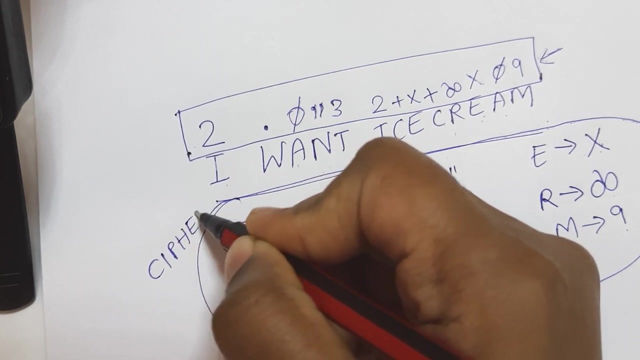 two means what? dot means what. this symbol means what? okay, only when you share this particular thing, okay, with your friend, only then he will or she will understand this particular message. Now, what do we call this particular coding, as we call this as cipher? okay, it is this. 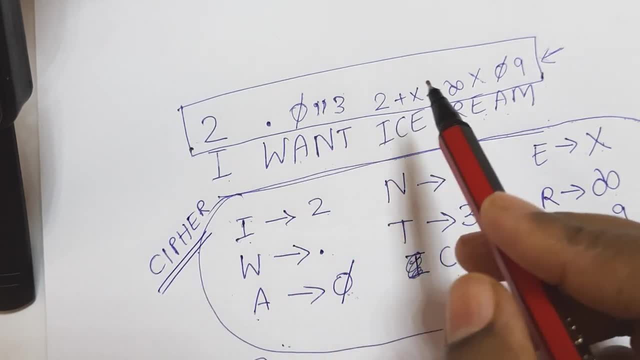 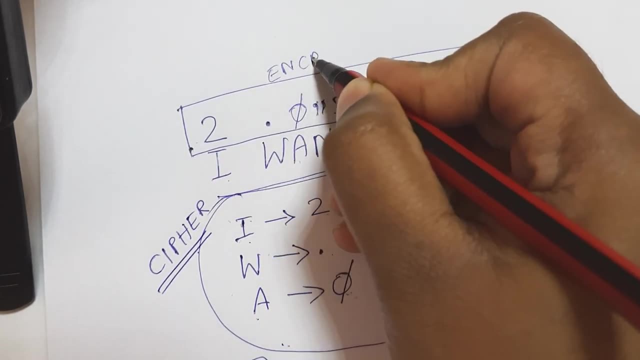 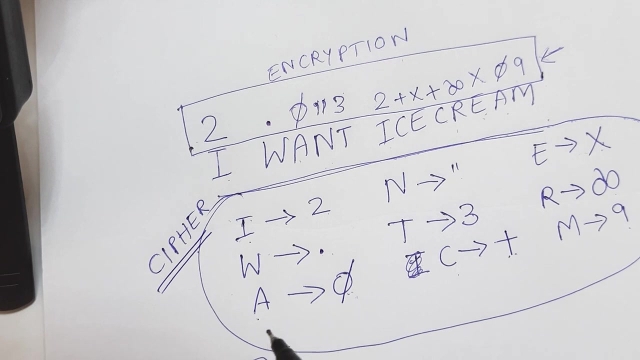 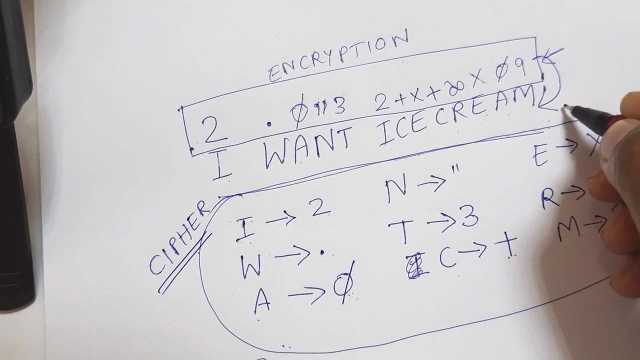 one which actually tells us on how to read a secret message. and do you know what this message is called? This is called as encryption. you are going to encrypt a message and make it into a secret message, And converting back from this message to this message is called decryption. 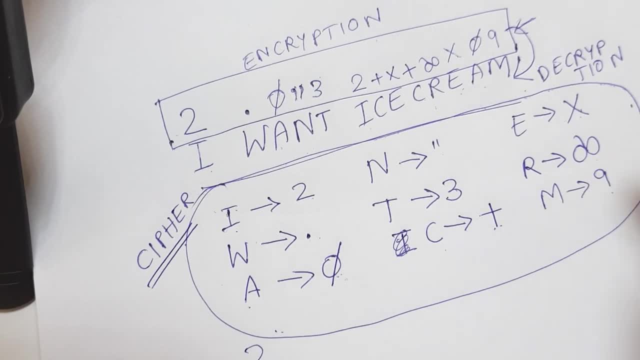 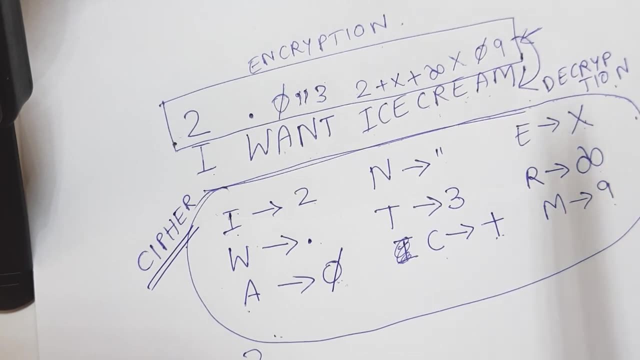 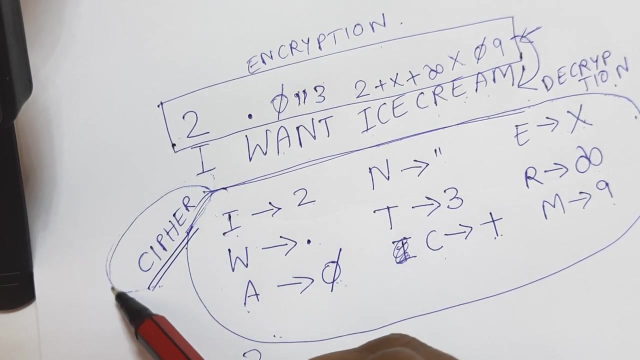 It is called decryption. okay, so the concept that we are going to learn today is something called as encryption and decryption, And what is the most important thing for that? it is the cipher, which actually tells us on how to convert Any message. 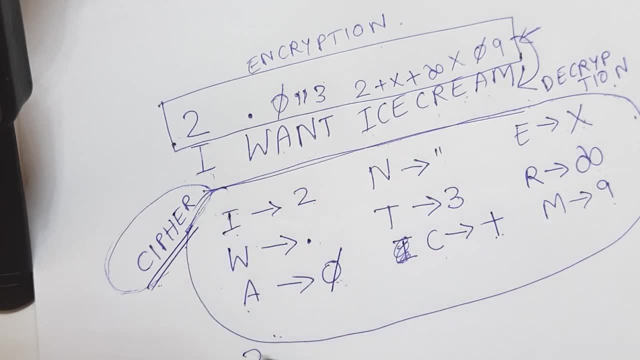 Any message in a secret message. So over here I have created my own cipher to convert it into a secret message. But let me tell you there are some standard ciphers which are there, which you don't have to share it with anybody. everyone will be knowing those ciphers, okay, but there are. 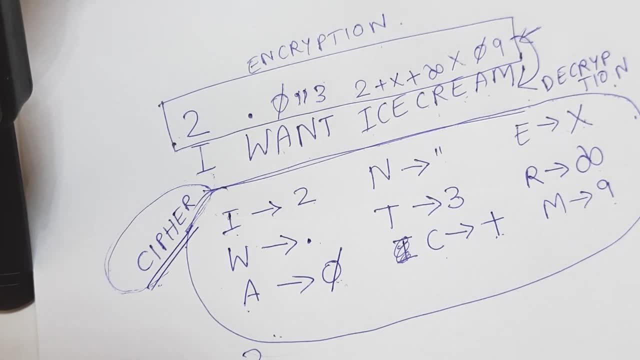 hundreds and thousands of ciphers, so people will not know which cipher they have to use for converting this message. so that way you can actually send any secret message to your friend. okay, Now let me just show you one of the kind of encryption that can actually be used for sending. 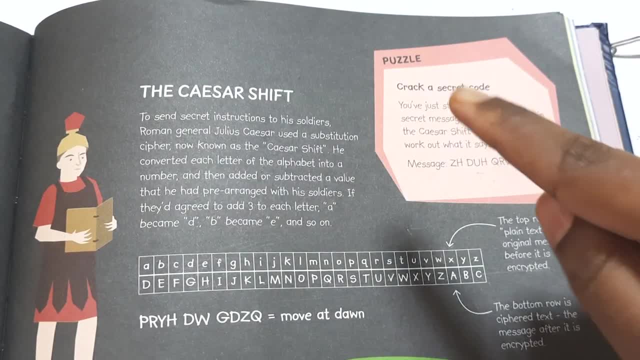 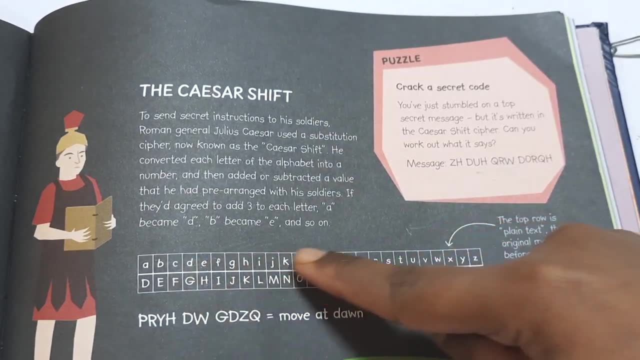 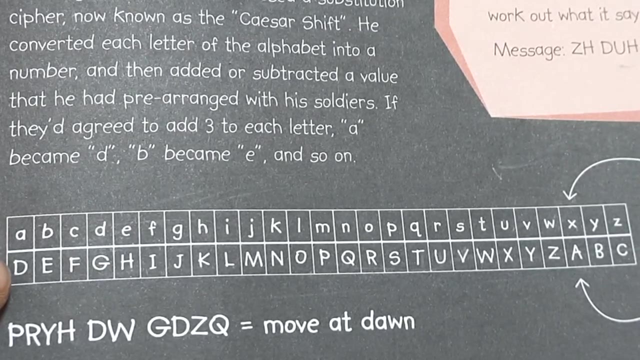 secret messages. Okay, so this one is called as a Caesar shift. okay, and this is the cipher. so basically, what this cipher means is: wherever you find A, you have to put capital D there. wherever you have small b, you have to put capital E. 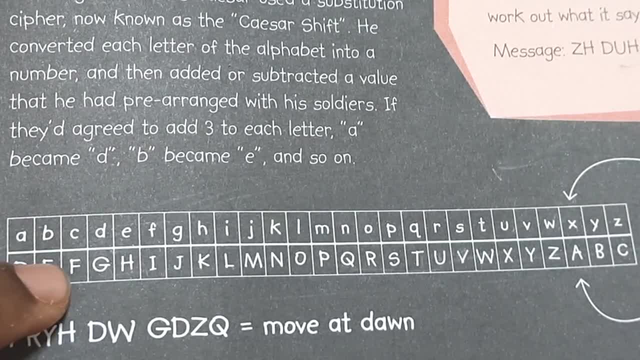 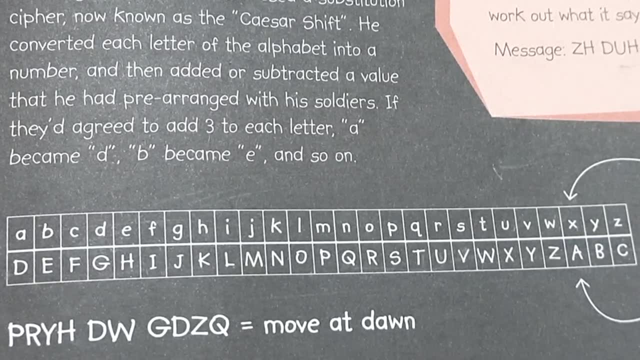 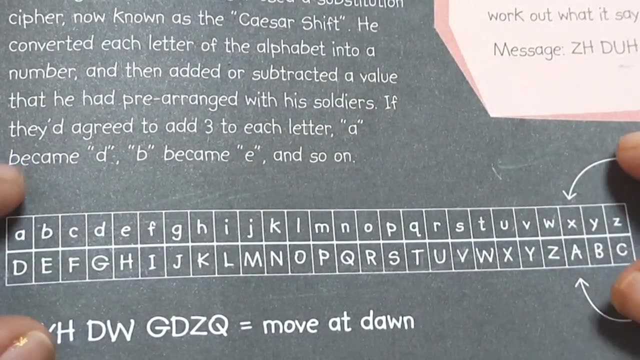 Wherever there is C, replace it with big F. okay, So like this, you will have to replace your message using these alphabets instead, rather than using symbols and numbers. they have kept it very simple, and this is very, very interesting, okay. 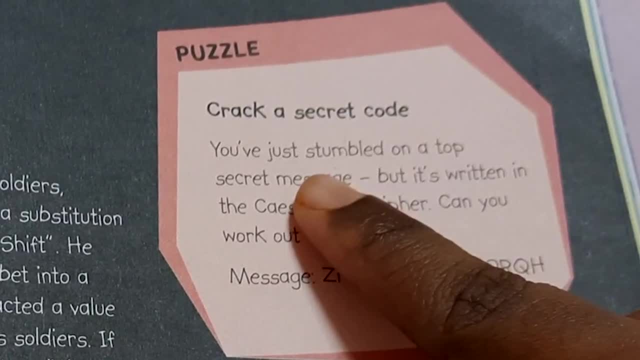 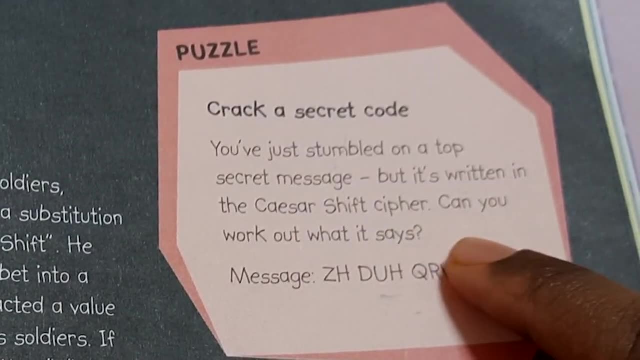 So let me just show you. they have also given a puzzle over here. So it says: you have just stumbled on a top of a secret message, but it is written in Caesar shift cipher. Can you work out what it says? So over here they have already given you a secret message. okay, but you will have. 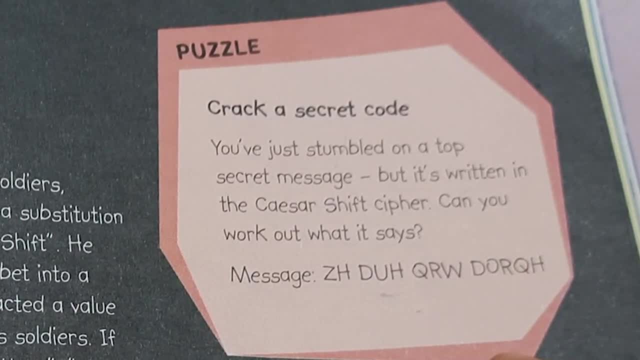 to convert it and you will have to tell what is the correct meaning of it, which means this is the encrypted message. okay, encryption is already done. they have already applied this and they have written a message. now you have to go back and get the secret message. 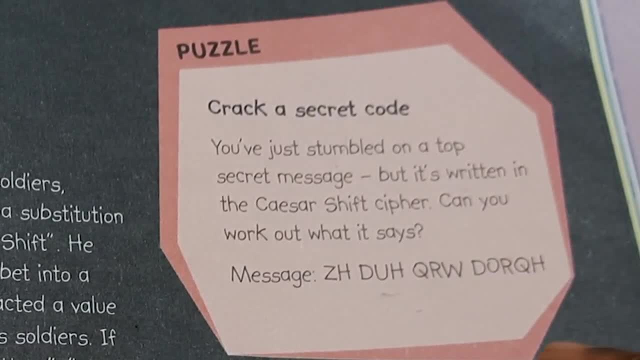 from this. so you have to say what the secret message actually means, and that is called as? What is it? Decryption? yes, you are right. okay, Now let me just write a simple sentence and I will show you on how to convert it into. 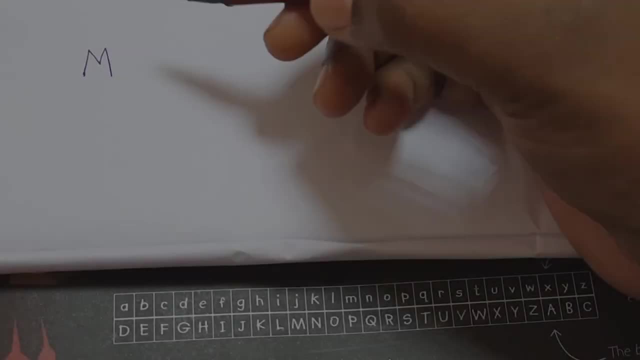 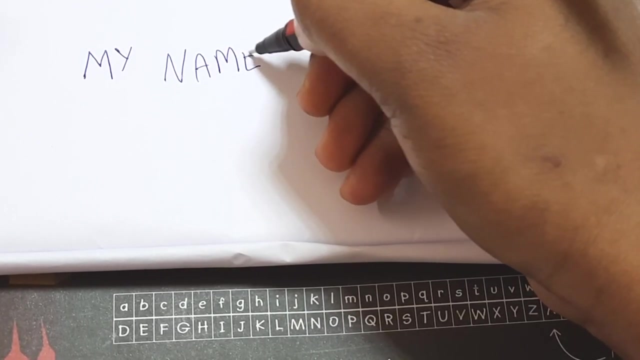 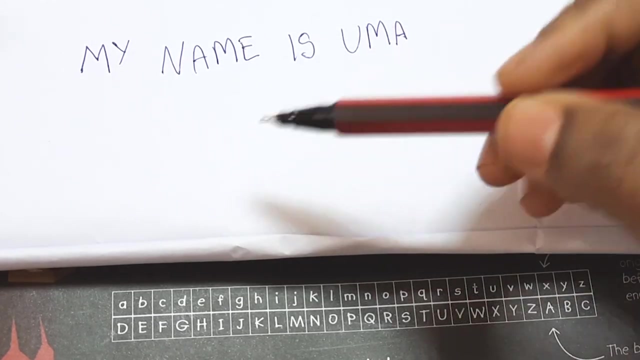 a secret message using Caesar's shift. So the sentence that I want to write is: my name is Uma. okay, So I want to use Caesar's shift. So I want to use Caesar's shift to actually convert this into a secret message. 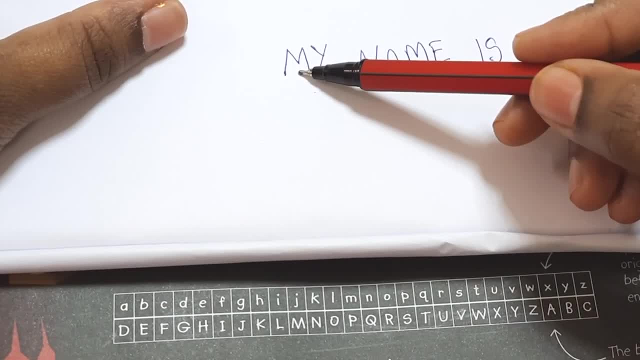 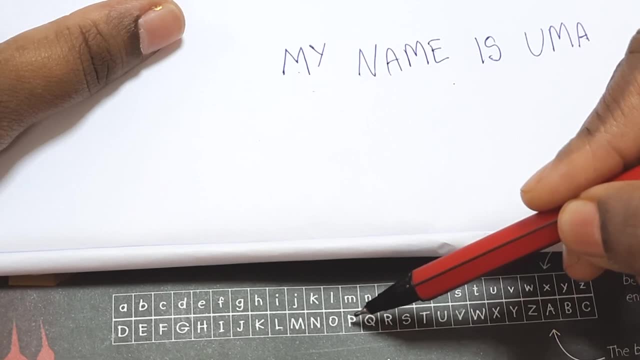 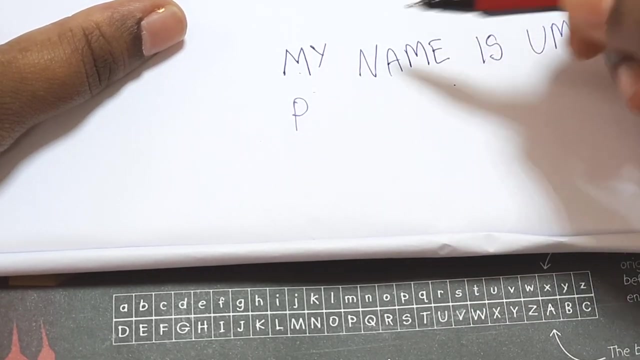 So how do I convert it? Now? the first alphabet is M, so we will have to search where is M in this. there it is. so what is there just below M? Oh, it is P. so instead of M I need to write P, and the next alphabet is Y. so where is? 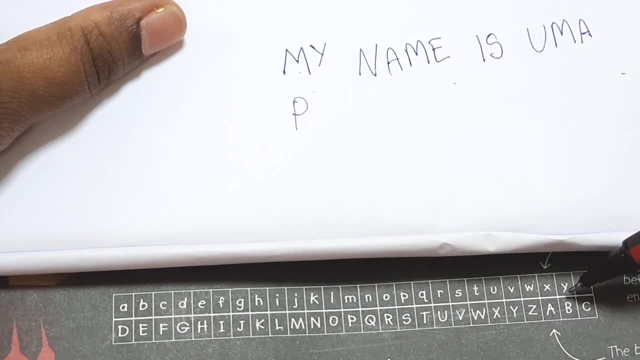 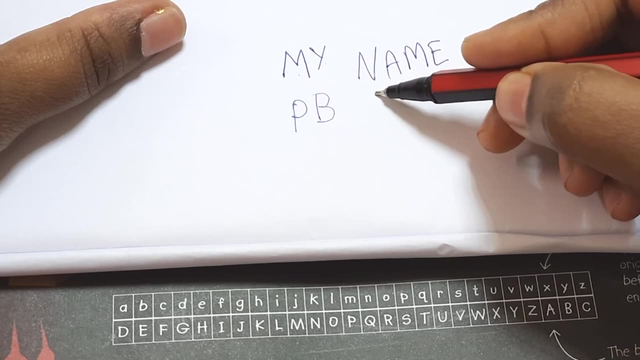 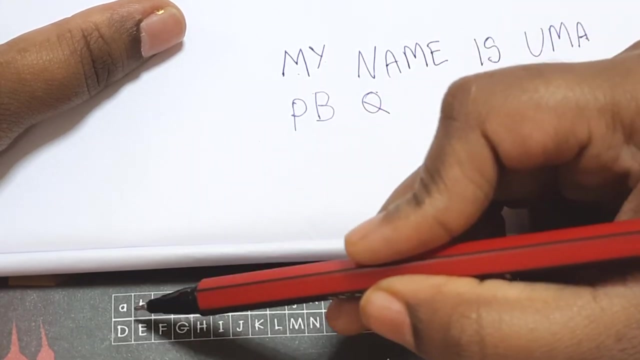 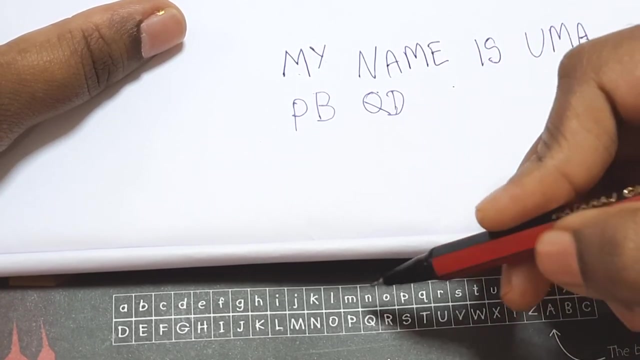 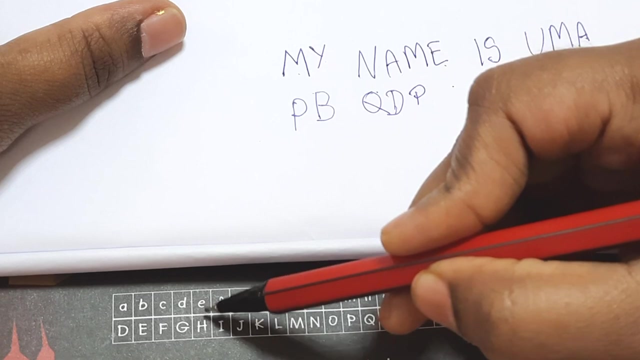 Y, Oh, here it is, So under Y it is B. Okay, So I need to write B, Now N, so under N I have Q, now it is A, under A it is D, then it is M, so under M it is P again, and now it is E, so under E it is H, now it is I. 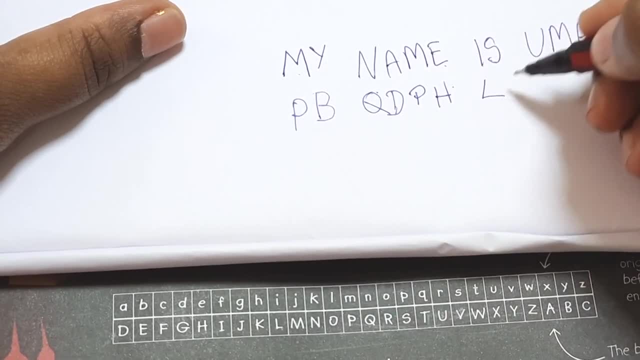 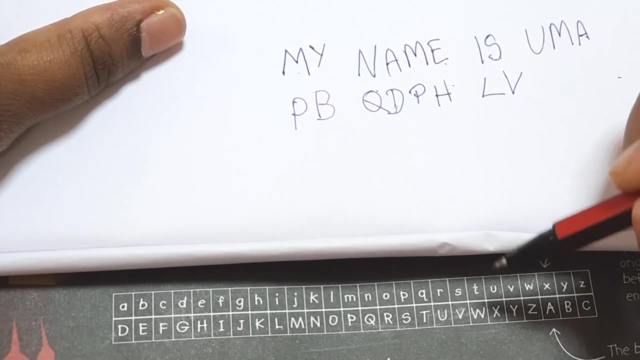 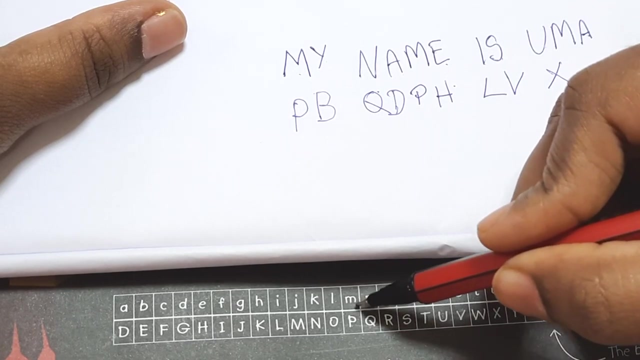 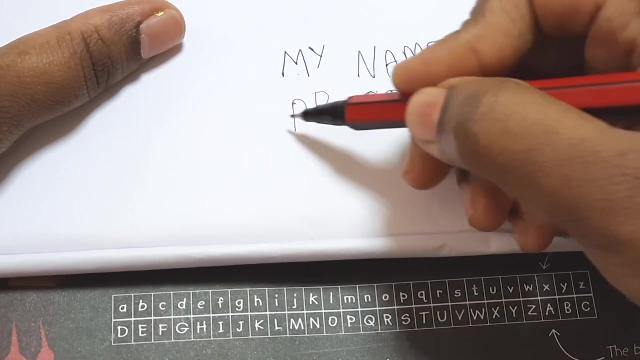 under I, it is L, the next is S under S, it is V, next is U under U, it is X, next is M under M, it is P, and last is A under A, it is T. so if I have to tell my name to somebody, 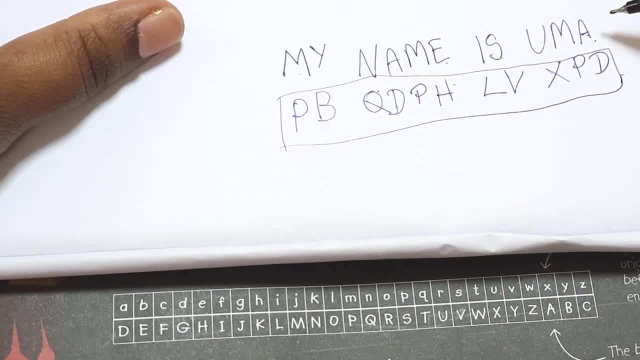 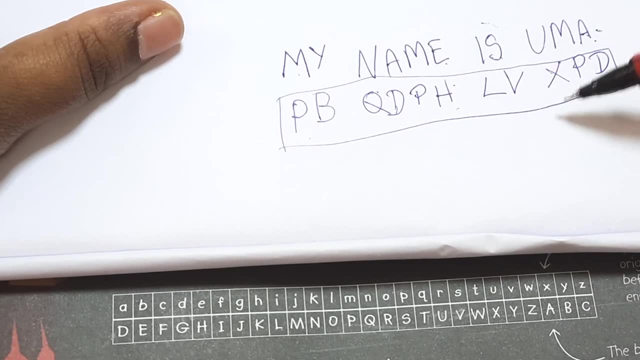 and I have to tell it secretly. Then, using Caesar's shift, instead of sending my name as Uma, I can actually send a message: PB, QDPH, LV, XPD. Now who will understand what I mean with this right? 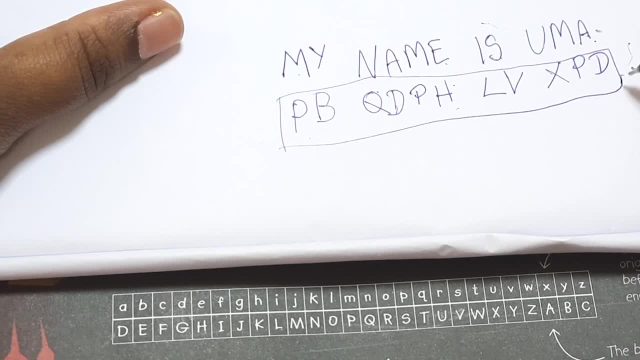 Unless they know Caesar's shift and they also understand that it is Caesar's shift that I have used to do it. I can use any cipher, I can use any method to encrypt it, right? So this is how easy it is to send a secret message. 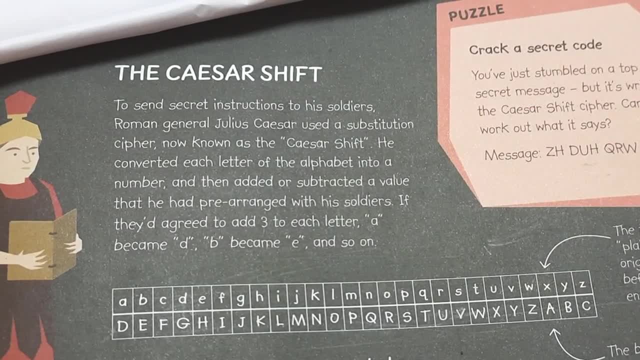 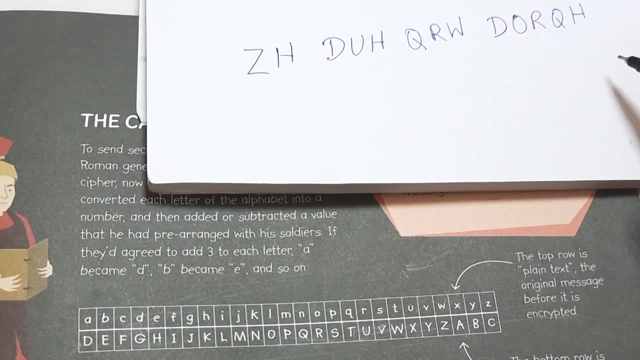 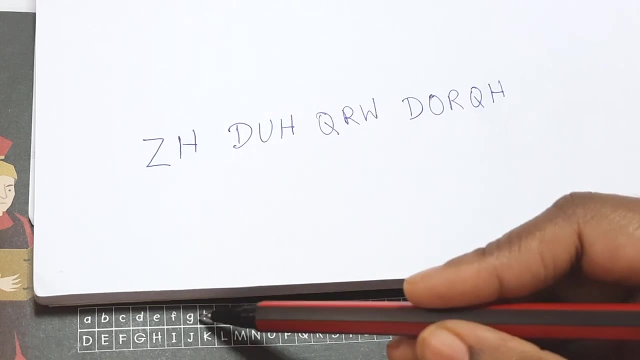 Now Shall we do this puzzle which they have given to us, So let me just copy this. okay, So this is the secret message. Now, what we need to do to get the actual message, We need to decrypt it, which means we should not search for the alphabet in the first line. 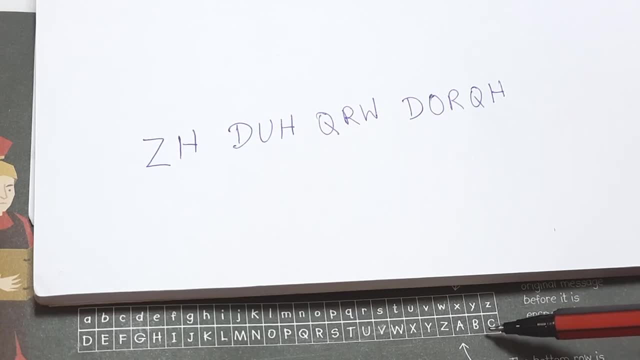 We should search for the alphabet in the second line and then replace it with the first line. That will be decryption. For encryption, you search it in the first line And then replace it with the second line. But for decryption, search it in the second line and then replace it with the first line. 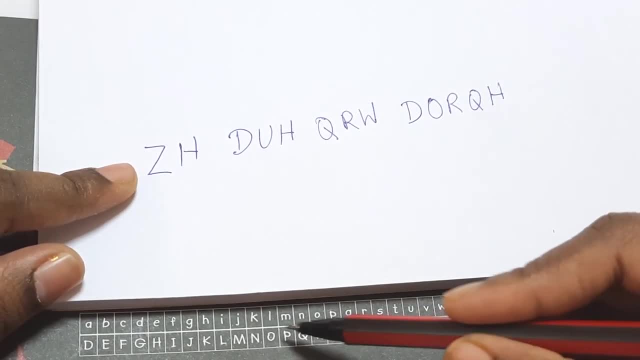 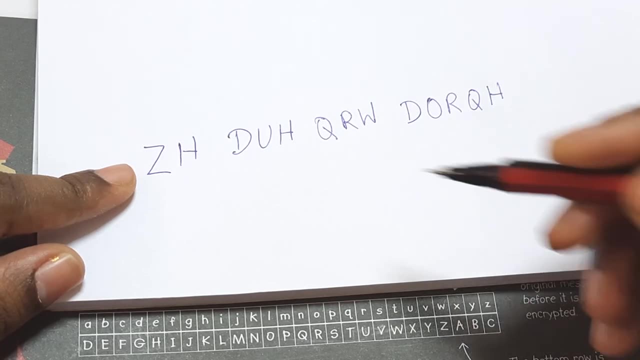 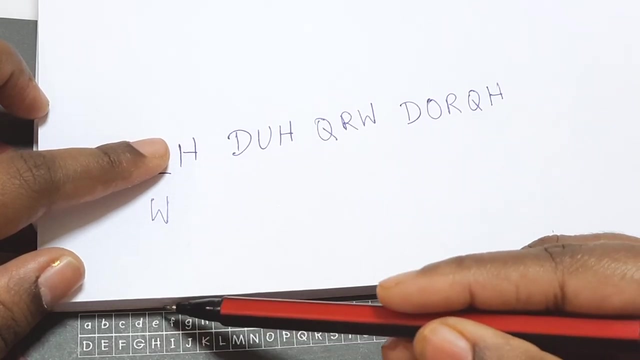 So the first alphabet is Z, So over here, if I search Z, this is where Z is, And for Z, the alphabet which is given is W. The next one is H. So where is H? Oh, H is here, So instead of H I need to write E. 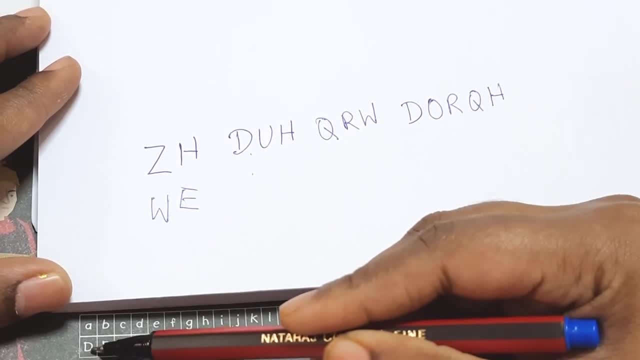 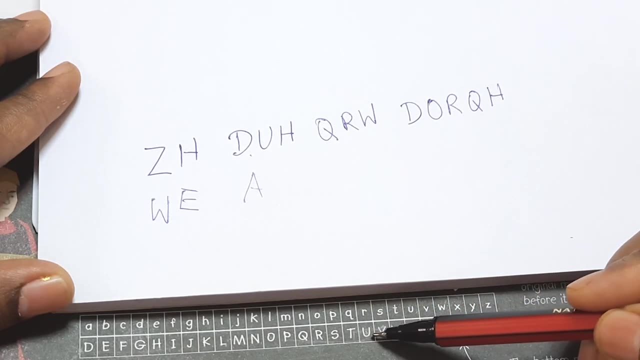 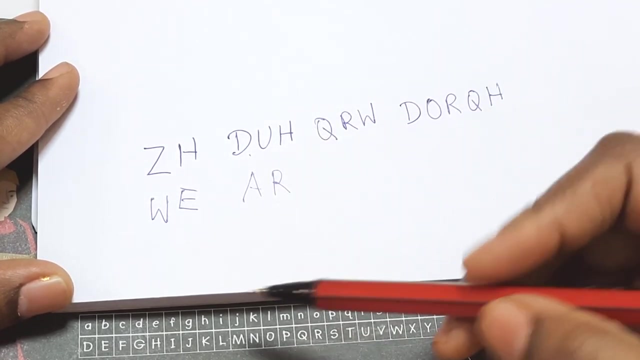 Now the next alphabet is D, So D is here, So instead of D I need to write A. Next is U. U is here, So instead of U I need to write R. And the next is H. Where is H? 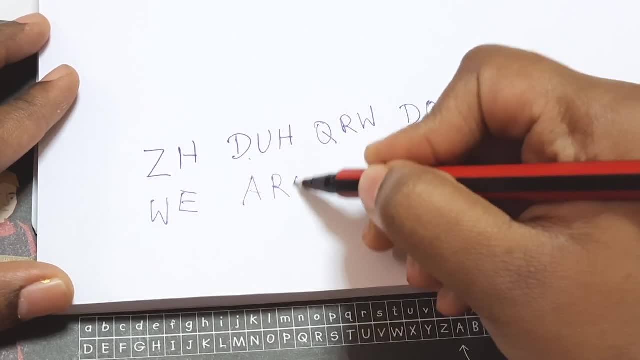 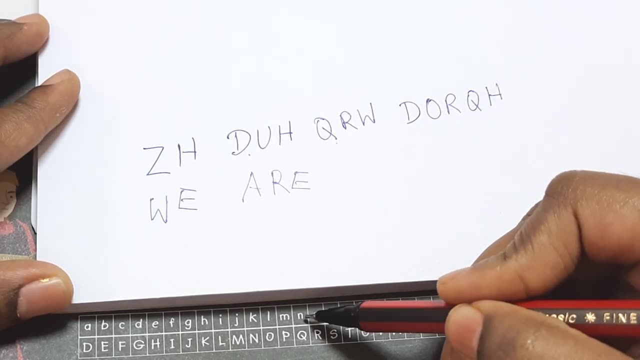 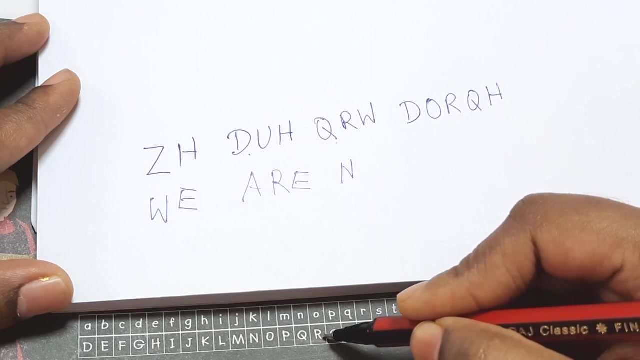 H is here, So instead of H, I need to write E. And the next alphabet is Q. Instead of Q, I need to write M. Then is R. Instead of R, I need to write O. Next is W Instead of W, I need. 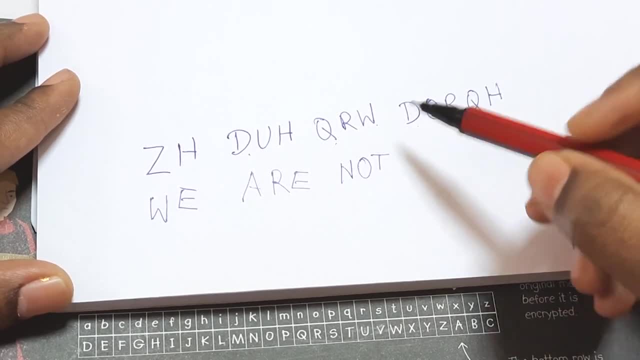 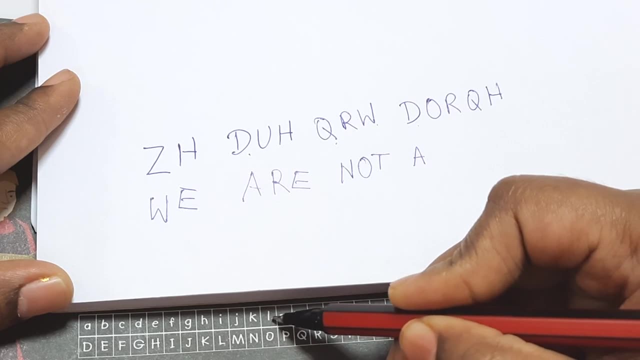 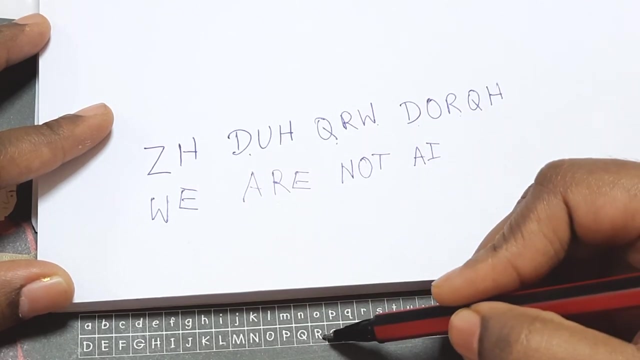 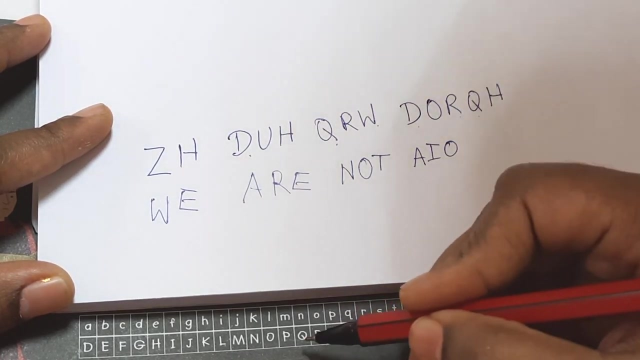 to write T, Next is D, D means A. The next is O. Instead of O, I need to write I. Then is R. Where is R? R is here, R is here. So instead of R, I need to write O. Then is Q. Instead of Q, I need to write N And the. 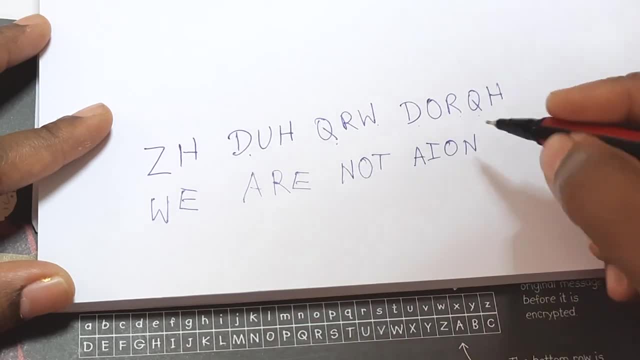 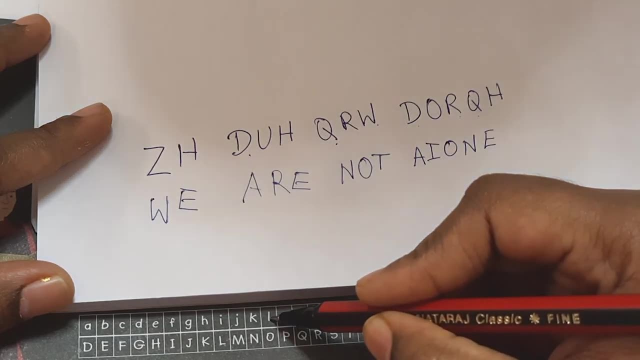 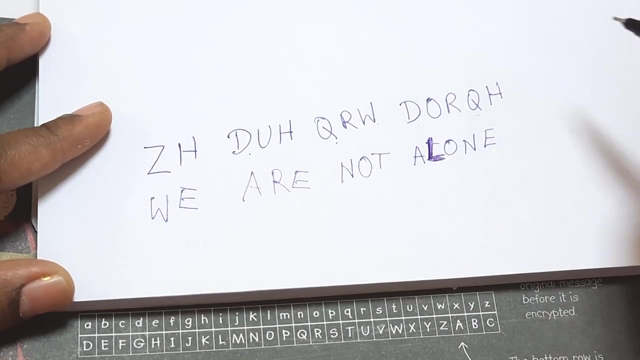 next one is H. Instead of H, I need to write E. I think I have made a mistake. So instead of O, I need to write L. It is not I, It is L. Okay, So We are not alone. 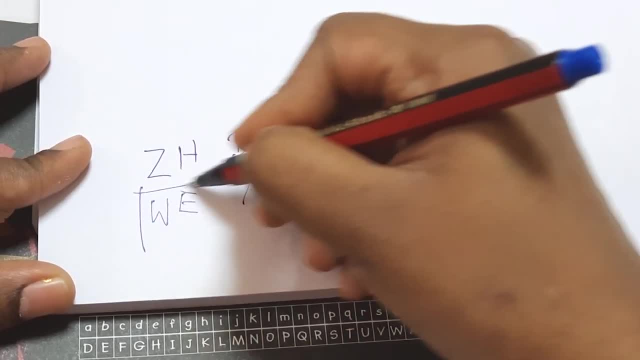 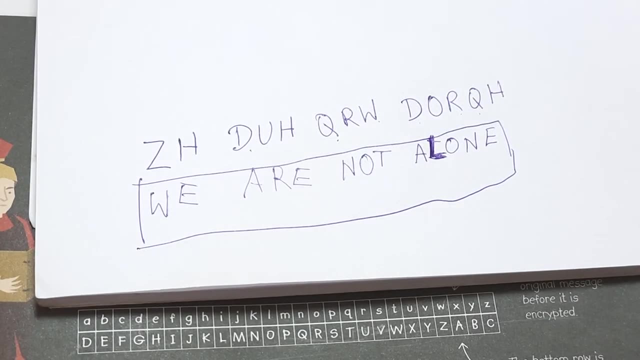 Yes, So the message- secret message- which was sent to me is that we are not alone. Oh my God, I think there is a thief inside the house. We are not alone, So please be careful. That is the message which is being sent. 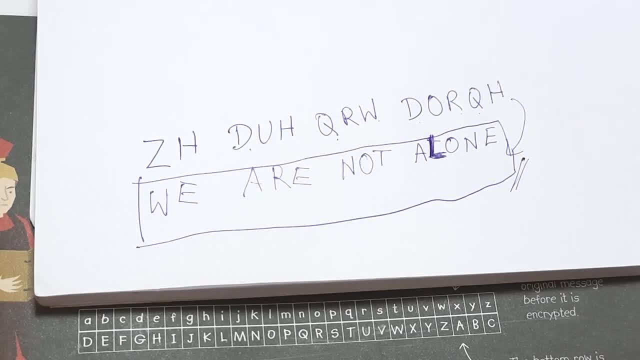 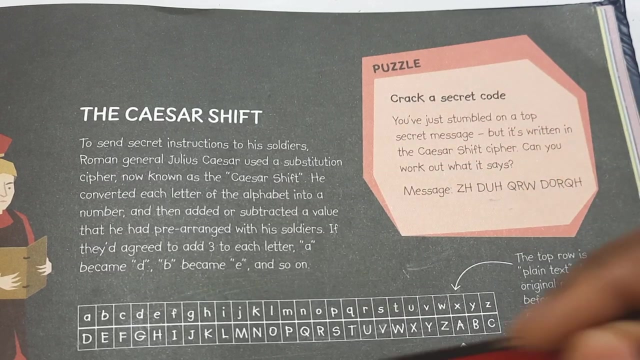 Now do you understand on how to do a decryption, And don't you think this is very, very interesting? Yes, So this completes today's video. So now what I'm going to do is I'm going to take a picture of this particular Caesars. 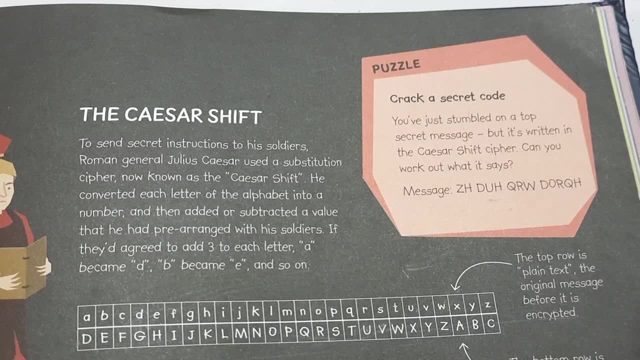 shift and I'm going to share it in the community page of my channel. So ask your parents to show the community page or to take a printout for you and to share it with you, And I will also be giving you some homework Now. this homework is going to be very, very interesting. 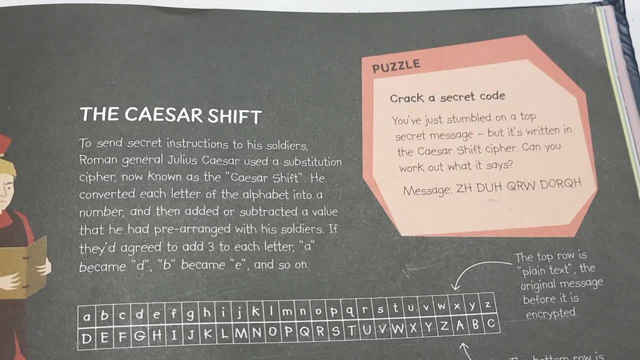 Okay, Because I want you to send me secret messages so that I decrypt it and send it over to you. I'm going to be using Caesar shift, Okay, So you have to send me secret message and put it in the comment on my community page.